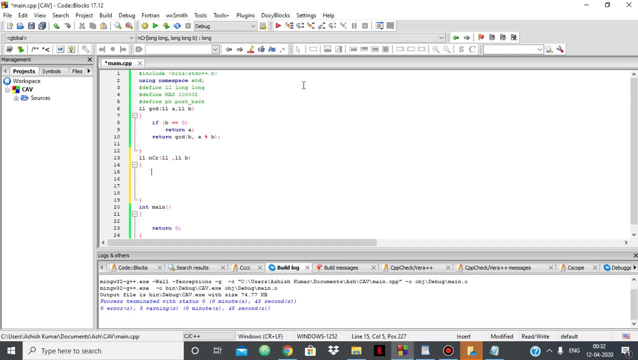 Hello everyone. in this video we are going to see how to find the value of nCr efficiently. So, as you know, nCr is basically n factorial by n-r factorial into r factorial. So for smaller values of n you can have a function factorial and you can find the answer using that only. 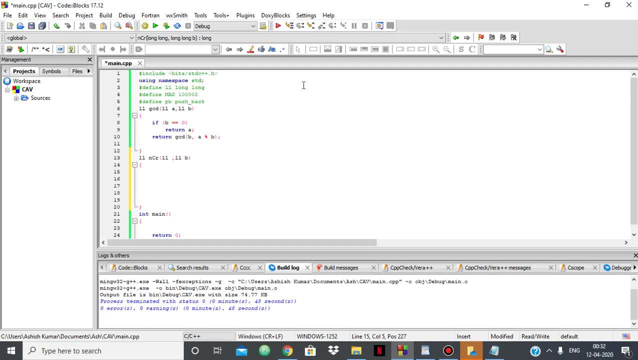 But for larger values of n. doing that will result into overflow. I recently faced this problem while doing a question on code forces. So in this video we are going to see a very efficient method of doing this, Which will simply make use of the fact that nCr is in the last. 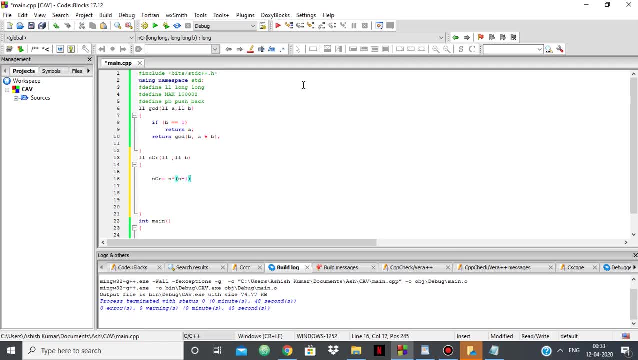 It is n into n-1, into n-2.. And till n-r plus 1. Multiplicated Why? Because r factorial will get cancelled By r into r-1.. All the way till r becomes 1.. So we have a product on the numerator, we have a product on the denominator. 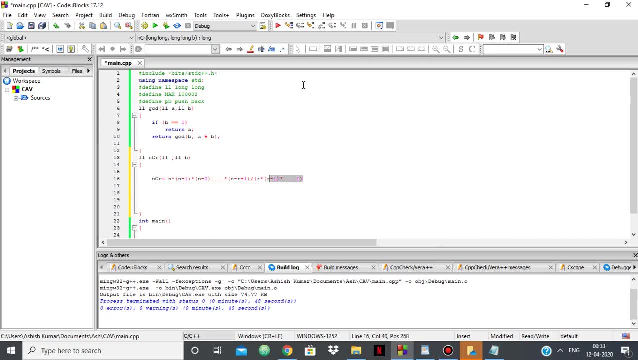 So at each point for multiplying- we will keep on simplifying it- We will find the GCD of n and r and we will divide the top and the bottom with that. Again, I will find the GCD of n-1 and r-1 and I will divide the top and the bottom with that. 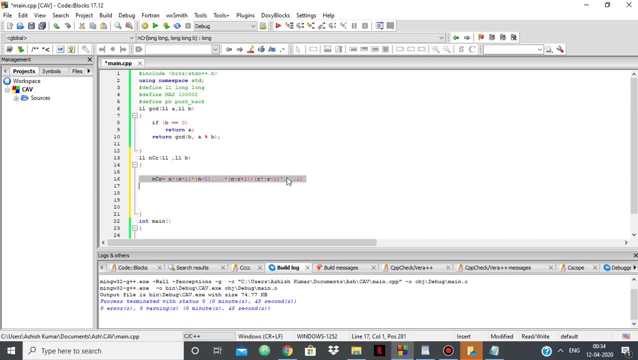 I will find the GCD of n-2 and r-2 and I will divide the numerator and the denominator with that. So I found this method on GeeksforGeeks and it's really easy and simple. So let's get to it. 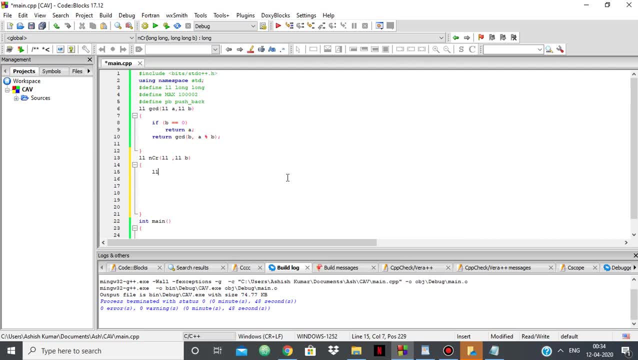 For the implementation I will be taking. let's just say ll. I will be taking. this is n and this is r and cr. So I will be taking a is equal to 1, b is equal to 1.. So a will be holding my numerator, b will be holding my denominator. 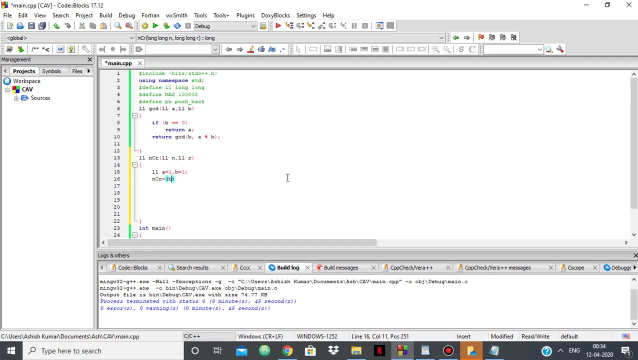 Now you should also know that ncr is equal to ncr-1.. So it's basically the same thing: ncn-r, my bad ncn-r. So ncr is the same thing as ncn-r, So we will be taking the smaller value of that. 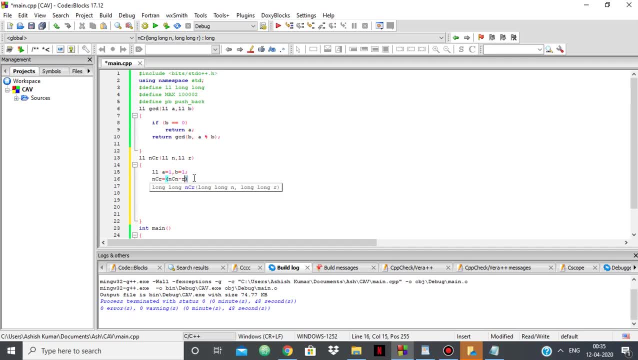 So if r is smaller than that, if n-r is smaller than that, So if n-r is smaller than r, then we will have that as r. Now, if r not equal to 0. Because if r is equal to 0, as you know, nc0 is 0.. 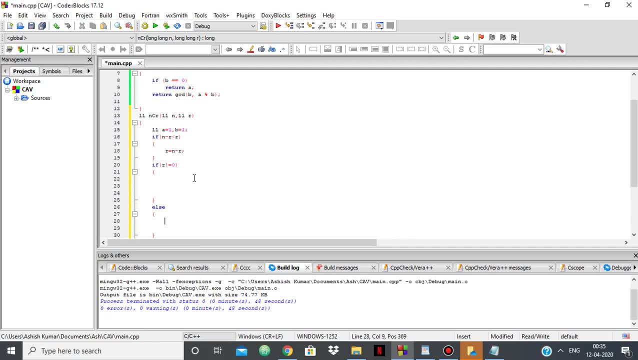 It's simply what: 1.. So if r is 0, then p will be our answer. Then p is equal to 1, simply. Otherwise, what we will be doing is we will go from r, like I showed before, The denominator will have r- into r-1.. 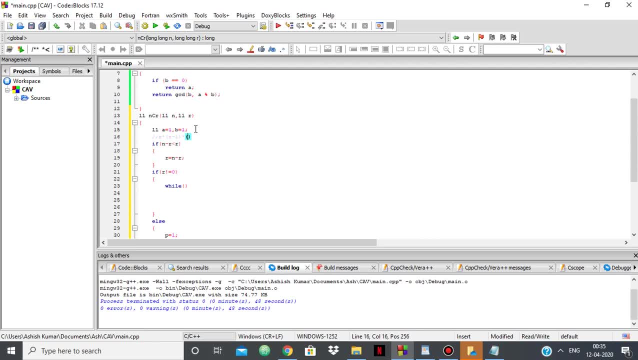 r-1 into r-2, all the way till r becomes 1.. So, while r is greater than that, What I will be doing is I will say p is equal to p into n And a is equal to a is equal to a into n. 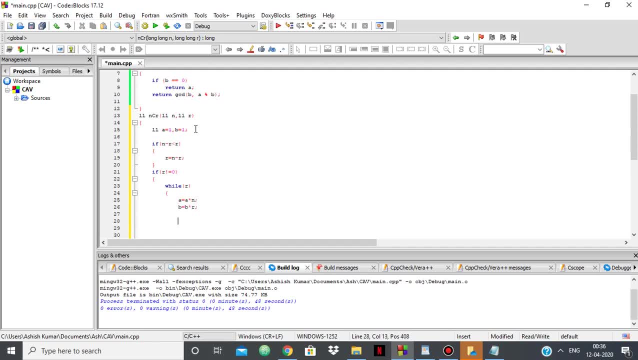 b is equal to b into r And, as I said, We will have a number for the gcd, So let's call it gcd itself gcd, Or let's say gc, Because we have a function called gcd. So llg is equal to gcd of a comma b. 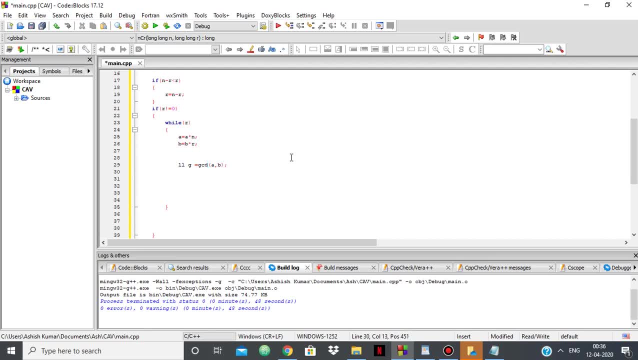 And then, as I said, we will divide the top and the bottom by that. So a is equal to a by g, b is equal to b by g, And then we will subtract n and r, Because it is on the top, n into n-1, into n-2, till n-r plus 1.. 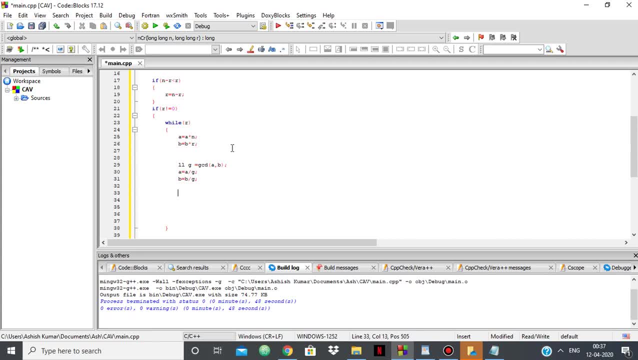 And on the bottom r into r-1, into r-2, till r, So n- minus r-minus, And so this will keep on going till r is equal to 1. And in the end we can just return p, Which will hold a final answer.